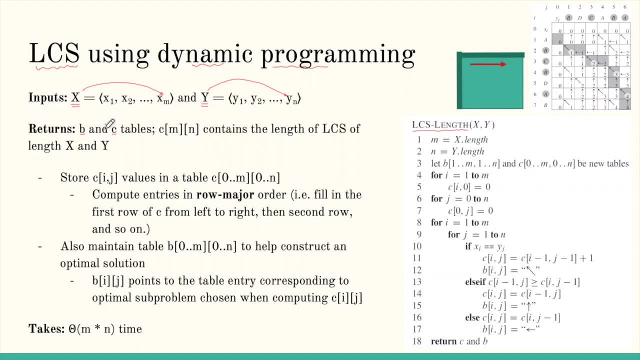 tables b and c. Now it's important that we understand what the purpose of these two tables are. The table ciz. this matrix contains entries such that ciz represents the length of the longest common subsequence so far. So ciz is the length of the LCS up. 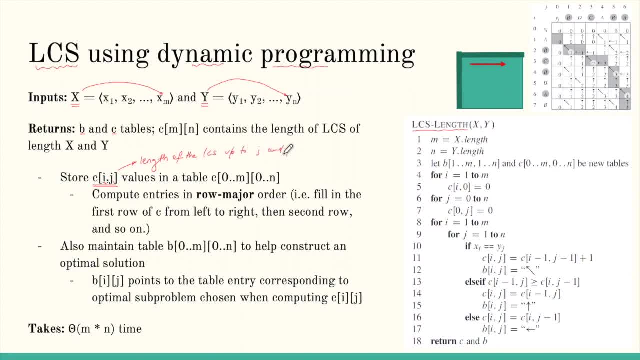 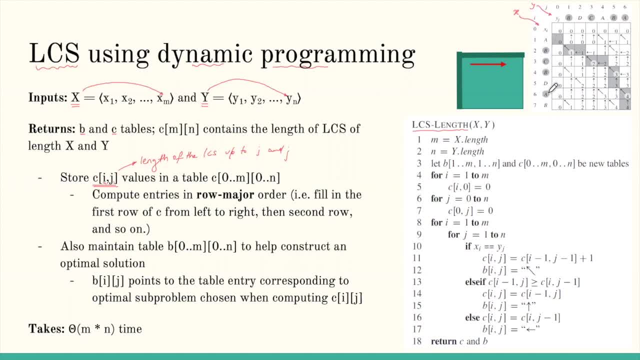 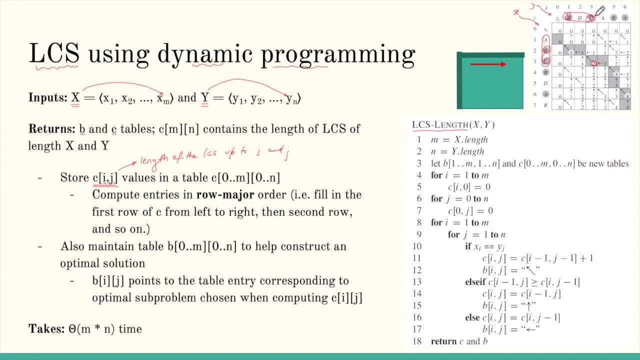 bc is the longest common subsequence. So in this way, at any point of time, ciz maintains the the length of the longest common subsequence. Now what the matrix bij represents is whether or not a given pair represents a part of the longest common subsequence. Now this matrix bij can contain. 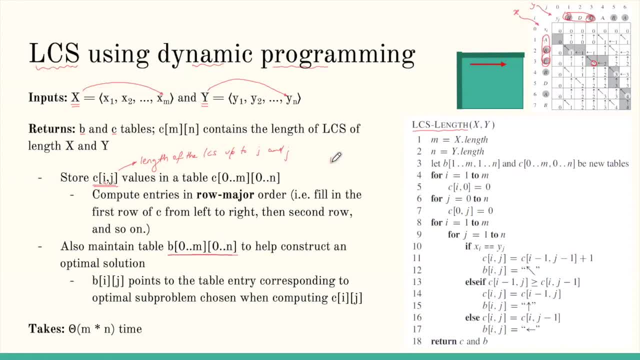 one of the three possible values: either the up arrow, or this kind of arrow, or the left facing arrow. Now, what this table contains once again is these particular symbols. These symbols- upward tilted arrows- represent the pairs which serve as a part of the LCS. Now looking at the diagram here for 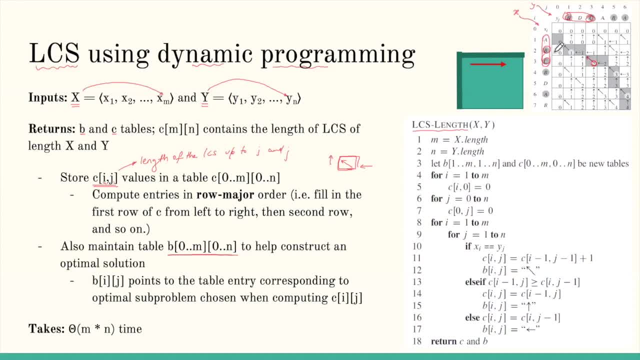 example, this arrow here says that in this sequence x, this character c and in this sequence y, this character c are a part of the LCS. So now at the beginning, we initialize c i 0 to 0 and c- 0- z to 0.. 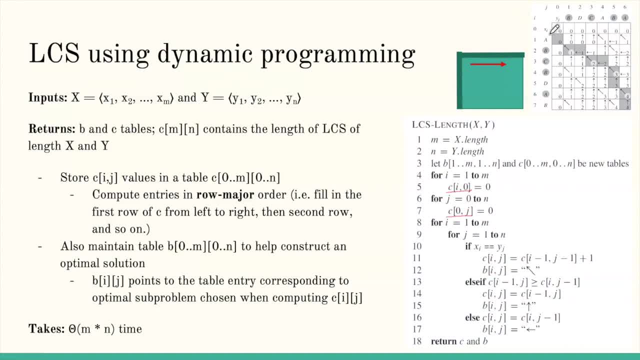 In other words, we want to initialize the LCS between our input sequence x with zero length y, as all zeros and our LCS between any length of y with zero length of x, also as zero. Now, following a bottom-up approach, we start with i equals 1 and j equals 1 and check if the two characters are same. 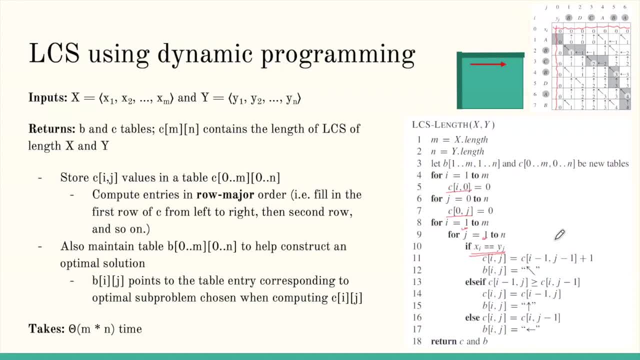 If the two characters are same, then what we simply do is we add 1 to the current LCS that we have. that is, the length of the LCS, to whatever the length of the current LCS that we have for the length i minus 1 and j minus 1.. Let's take 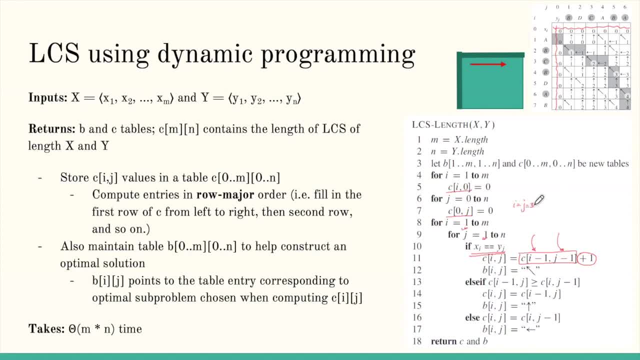 the example of i equals j equals 3.. When i equals j equals 3, that means we are at this cell, our x 3 is c and y 3 is also c. At this position we have x, i equals y j, because c equals c and 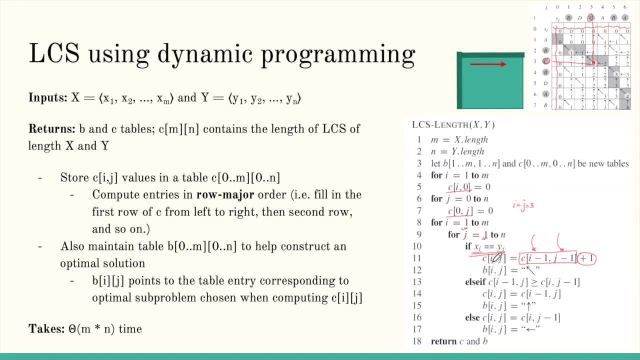 the way we calculate c i, j or c 3, 3 at this point is c 2, 2 plus 1.. So c 2- 2, what we have is 1, and then we add 1 to it, and that's how we get this 2.. And then we also set our matrix b i z to this tilted. 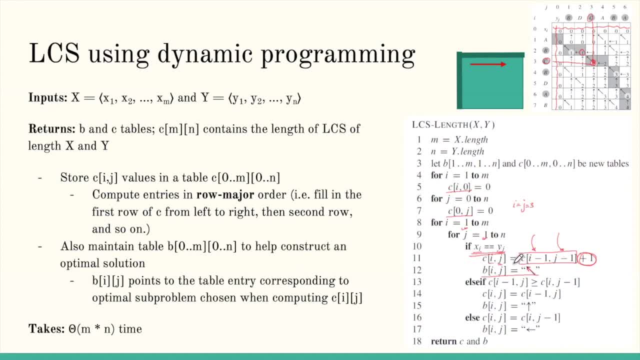 upward facing arrow, because this is one of the cases where we have x i equals y, j, and then this represents the common character that is a part of the LCS. Also, if you remember, this is also the equation that expresses the recursive definition of the LCS problem. To consider the next scenario, 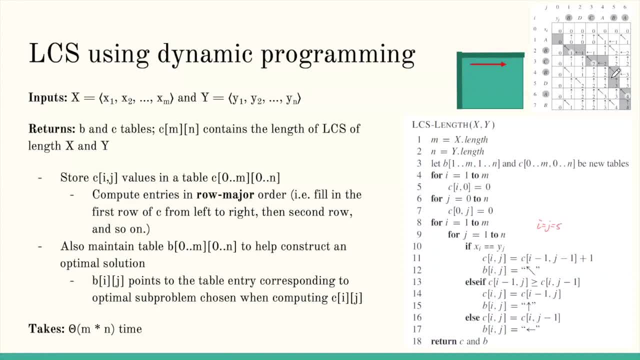 say, for example: i equals j equals 5. that is what we are looking at. is this cell right here? Then what we check is: is c i minus 1 j is greater than, equals to c i, j minus 1.. In other words, we are checking if c 4- 5 is more than or equals to c 5, 4.. So c 4- 5 will be this number here. 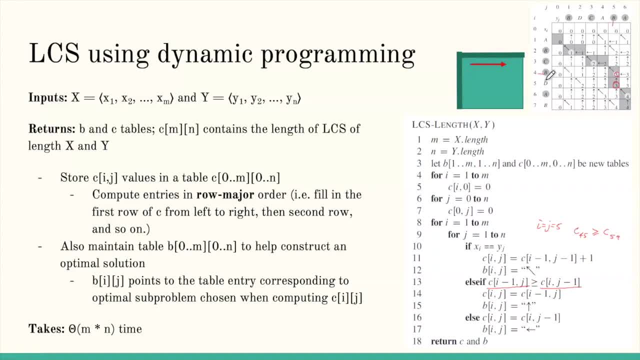 3, because this is c 4. 5 is more than or equals to, 3 is more than, equals to c 5, 4, which is 2.. So this is one of the cases where what we want to do is go up next step or like in a go, go, look for the next character in your sequence x. So here we set. 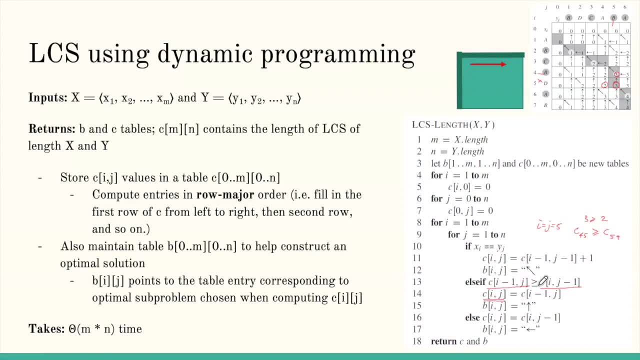 c i j, our current i j, will remain same as c i minus 1 j, that is, in this case c 5- 5 will maintain same as c 4- 5.. So in this case, the highest of c 4- 5 and c 5 4. this is 2. this is 3. 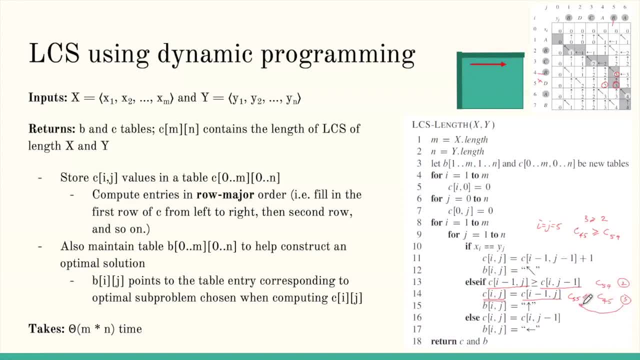 and the maximum of these two is 3, and this will go into c, 4, 5, 5.. Once again, this follows the recursive definition of obtaining the maximum between the two possible smaller values of i- j combinations. The next possible scenario is the last LCS statement and say, for example, when i equals 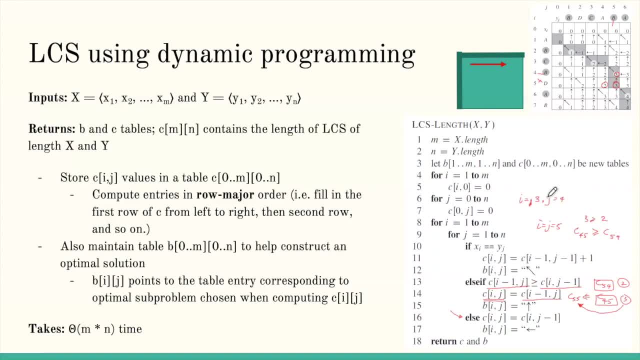 3 and j equals 4. what happens is we we know that in this case, c i minus 1 j is less than c i- j minus 1.. So in in such a scenario, we want to set: c i- j equals to c i- j minus 1.. In other words, here we want to set: 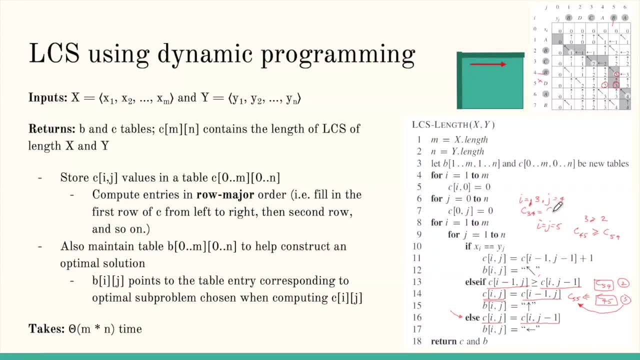 c 3: 4 equals to c 3: 3 and c 3: 3. here is 2, which is which becomes now the, also the longest common Length, and we also want to set this arrow to this side, suggesting that we are now going to look at 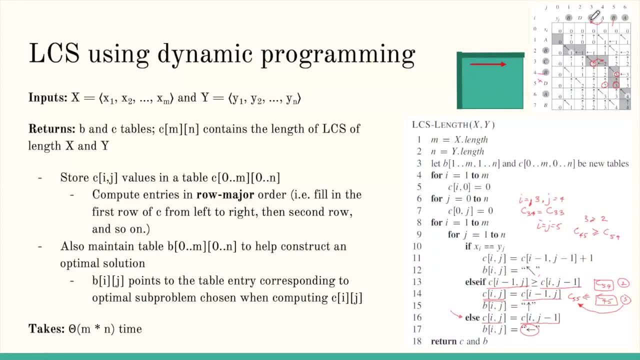 the next character in our sequence y. So finally, in the bottom of fashion, we continue this for loop and continue this execution from the top left corner all the way to the bottom right corner and at the end we return these two matrices, c and b, as our solutions. Now, because these for loops run, 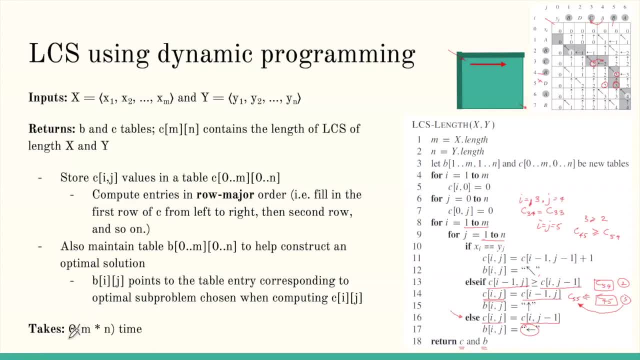 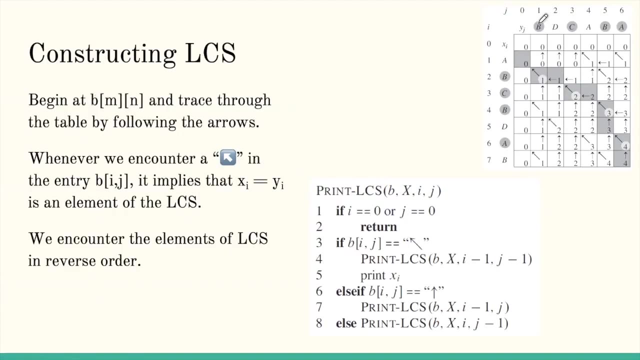 to m times n. the running time of this all rhythm is big theta of m times n, where m is the length of our first subsequence, x, and n is the length of our second subsequence, y. Now to print the solution of LCS, that is, to actually print the sequence b, c, b, a, we will need another function, print LCS. that takes 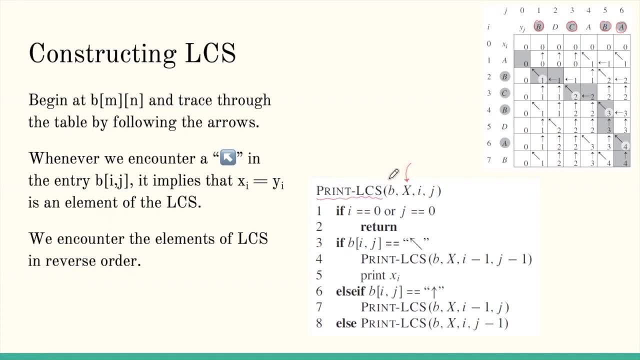 one of the sequences say x, our solution matrix b, and then we will need another function print lcs, and then i and j as the running lengths. So we call this function print lcs, passing the function b, m, n and also passing one of the sequences x and then providing i and j as their maximum possible. 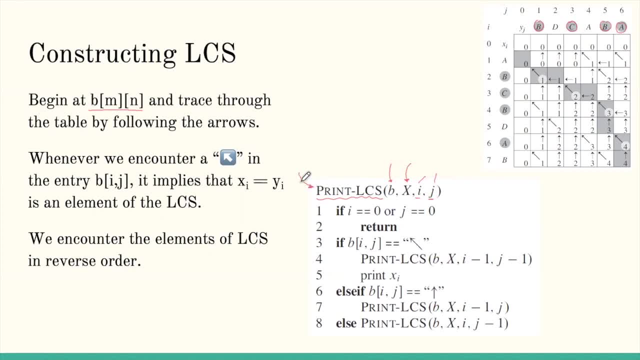 values. Now, this is a recursive function where we what what we want to do, is start from the bottom right corner and recursively navigate all the way to the beginning, um, or all the way to the position where we start, where we started making the first comparison of x. 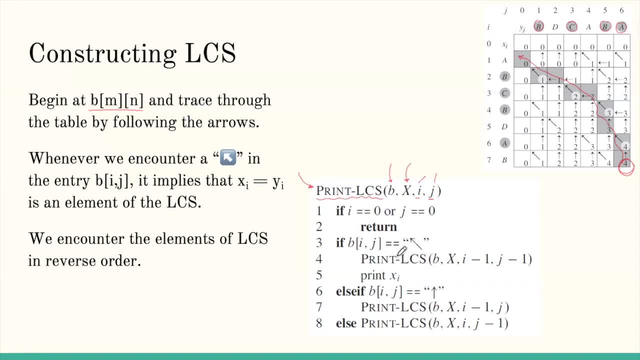 i and and y j. So this is the recursive function, where we start with i and j as their maximum values. we check if the solution has an upward facing arrow tilted arrow like this. If we do find something like this, that means that we have found the first possible. 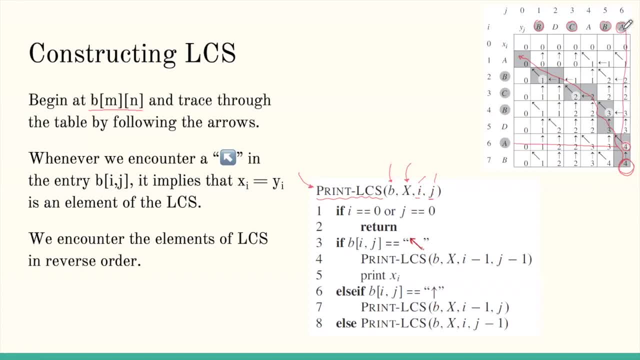 place where we have in a character in the LCS. So then we call the same function again by moving it one position, um up and left, that is um for a subsequence of length i minus one and j minus one, and then we do print xi. So since this is recursive function and we keep, 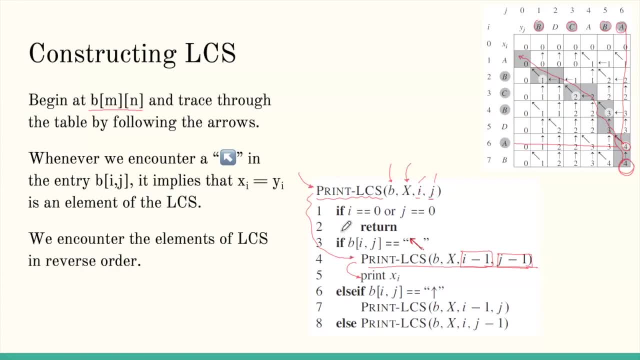 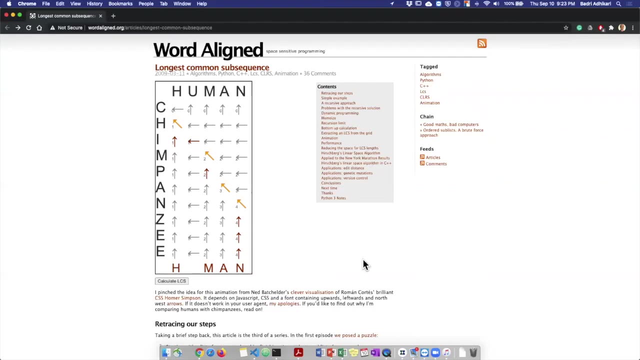 calling printed print lcs. with print lcs, the first character that will be printed is the first matching character and as the recursion winds back down, it will print all the characters subsequently. So the second question is: what is the longest common subsequence? Thomas quest has actually posted a really interesting article on longest common. 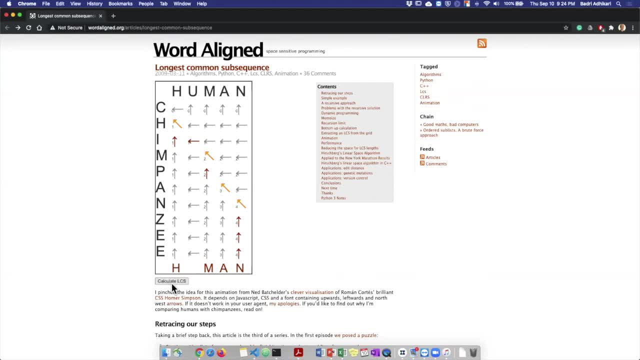 subsequence, and he also has a visual that shows how the algorithm actually works to calculate longest common subsequence. So here's a gif and image that shows how the algorithm calculates the values of the two matrices c and b, If you are interested more in this topic of longest common subsequence. 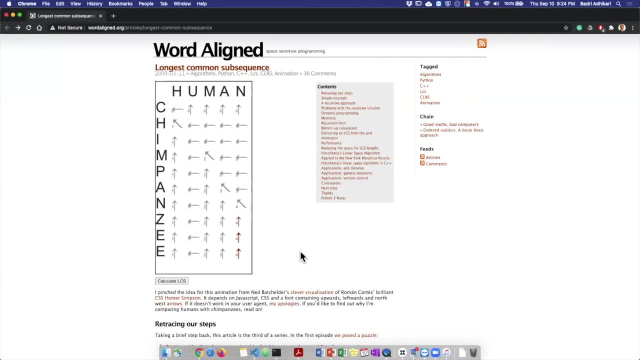 I encourage you to read this article and maybe even try some of the code that he has written.